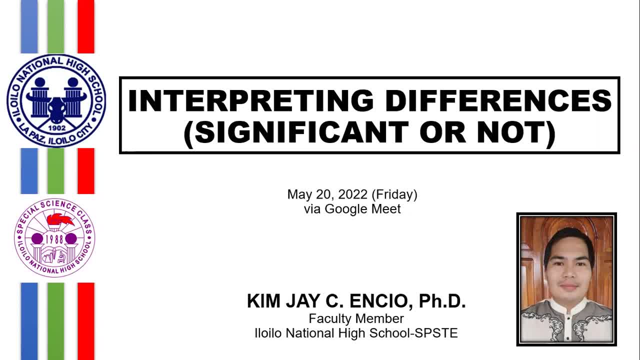 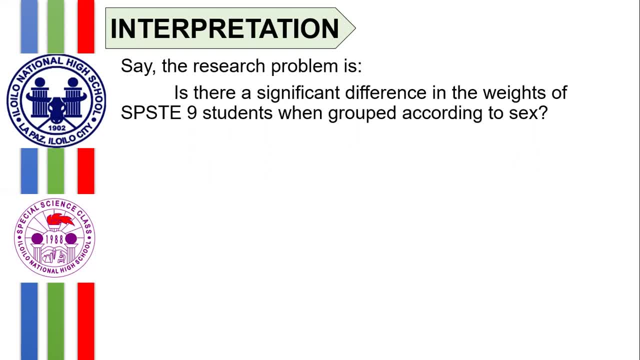 mean in the context of research. Basically, the research problem is: your inferential research question is: is there a significant difference in the weights of SPSTE-9 students when grouped according to sex? And your findings show that the mean weight of all the males is 58.59 kilograms, with a standard deviation of 2.5. 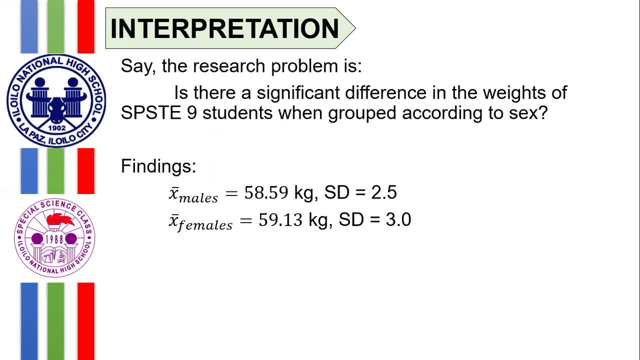 kilograms. The mean weight of the females is 59.13 kilograms, with a standard deviation of 3.0.. So you could see that the mean weight of the females is greater than is not equal to the mean weight of the males. However, after doing some sort of inferential, after doing your analysis, you are able to find out. 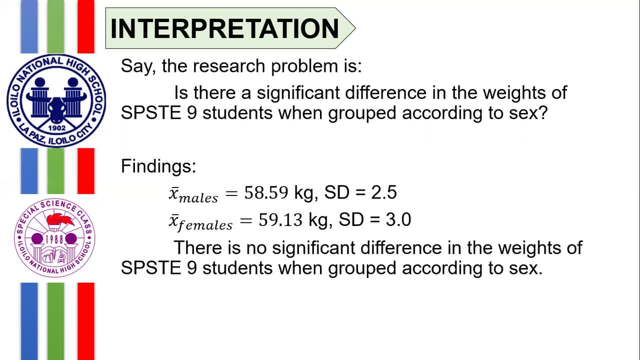 that there is a significant difference in the weights of the females And the mean weight of the females is no significant difference in the weights of spste9 students when grouped according to sex. so what does this mean if there is no significant difference between the weights of 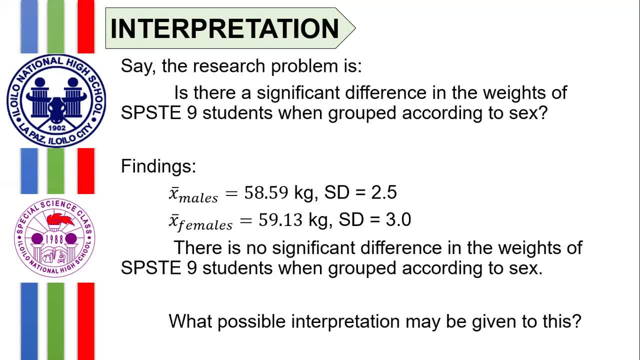 between a male and female's weights. what does that mean? what possible interpretation may be given to this? note that there are many ways of writing your answers and probably the way that you write your answer is different than mine, but what is more important is that the thought of the answer is correct. 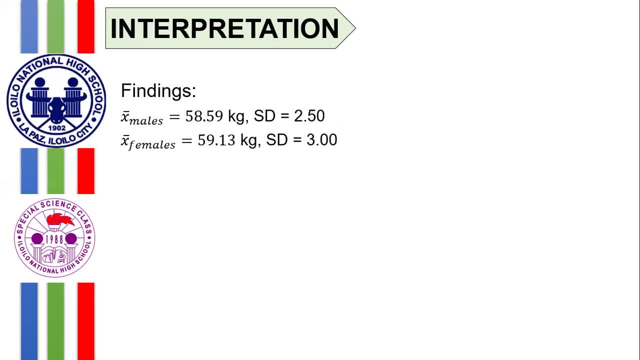 so remember, in statistics, if there is no significant difference between the weights here, so we are actually saying that they are statistically equal with one another, although in reality, if you would take a look, their mean weights are not equal. but since there is no significant difference between these weights, 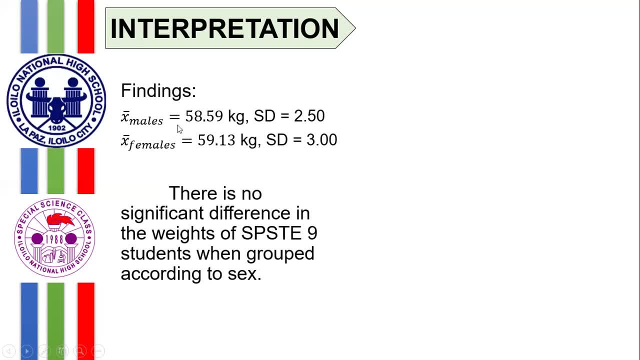 then there is a good reason for you to say that, statistically speaking, the mean weights of the males and females are equal with one another. hence, a possible interpretation may be this, and there are many ways to interpret this, but it is lots of reason for me to too, to not wear my only audience maile myожет, my books mygeht, and I hate it. I love you. 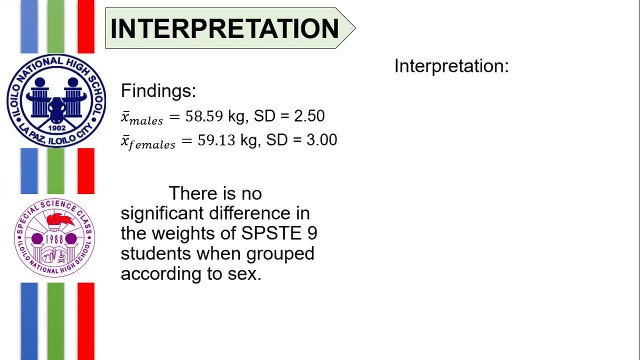 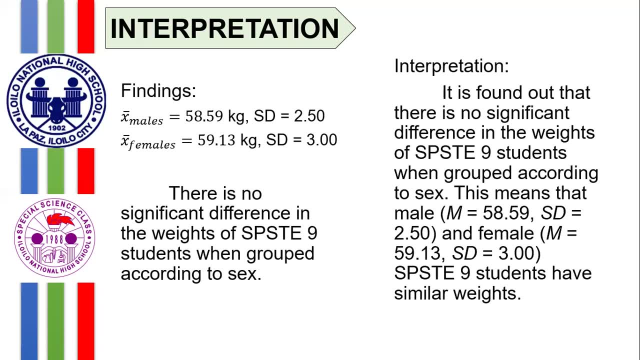 of reporting your answers, but for now we will stick with this type of reporting in class. It is found out that there is no significant difference in the weights of SPSTE 9 students when grouped according to sex, So I just really reiterated this. Then you provide an implication. 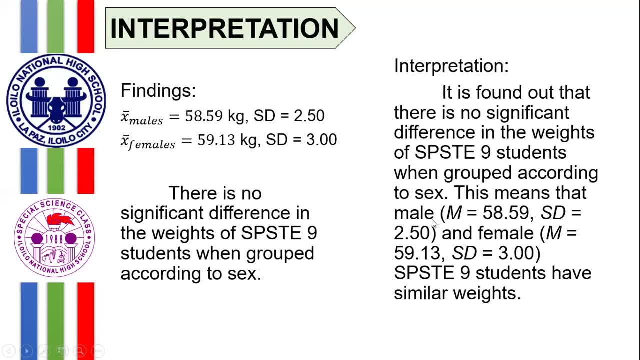 or a meaning for that. This means that male. then you copy the mean and standard deviation of their weights For the write-up. I want them to be in: M for mean and SD for the standard deviation That the males with. M equals 58.59 and a standard deviation of 2.50. 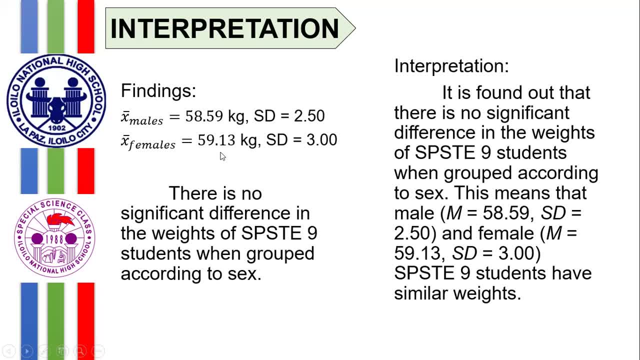 and female, with mean weight of 59.13 kilograms and SD of 3.0, SPSTE 9 students have similar weights, Meaning to say male and females are somehow similar mean and the mean weight of males and females are statistically equal or similar with one another. So that is the meaning of this. 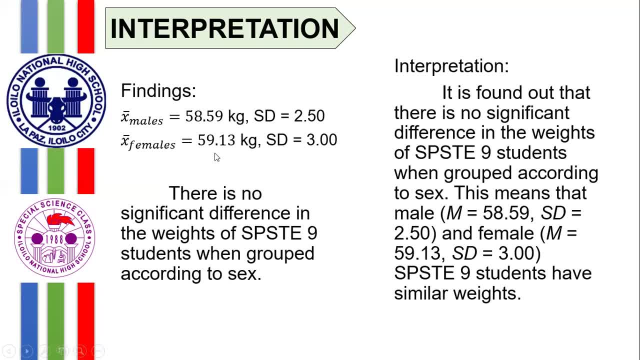 Although, analyzing the data, there is a difference really, but that difference is not significant. It's not big enough to be significant. That's why we treated them as statistically equal. that's why we come up with this interpretation. So that's the first one. How about if I give you? 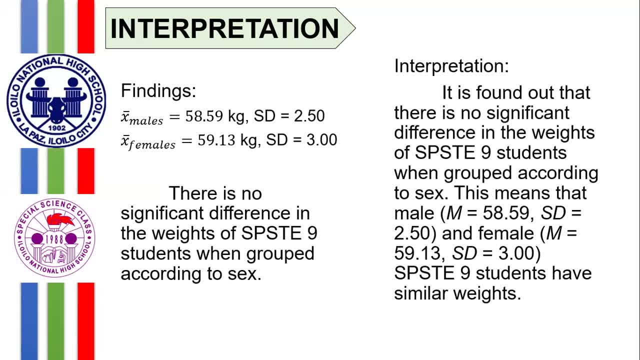 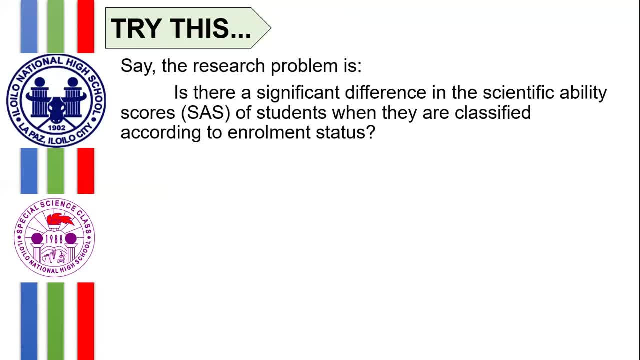 another one. Let's have another example, Say. the research problem is: is there a significant difference in the scientific abilities course, or SAS, of students when they are classified according to enrollment status? So suppose your findings- again these findings- are fictitious. but suppose your findings say that the mean scientific ability scores of the scholars are 75.45. 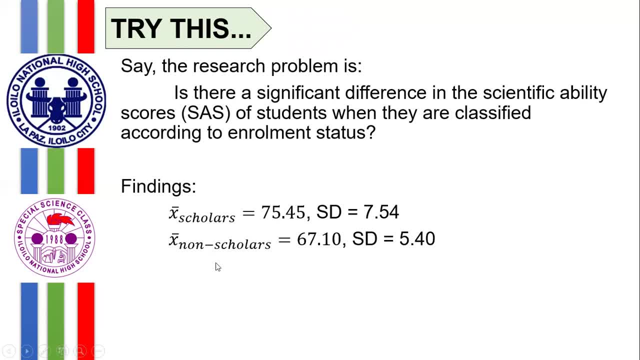 and with an SD of 7.54.. Whereas for non-scholars their SAS is 67.10, with a standard deviation of 5.40.. And suppose your statistical analysis showed that there is a significant difference in the scientific abilities course, or SAS, of students when they are classified according to enrollment status. 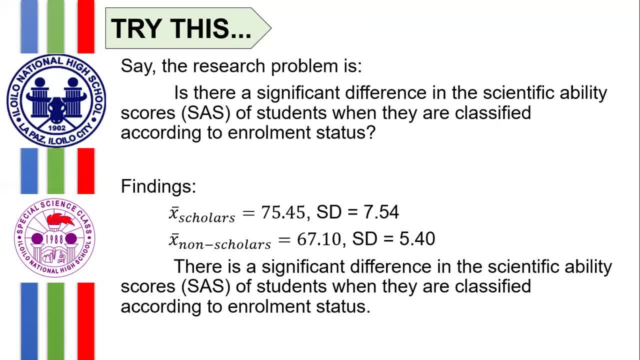 So this time the difference is significant. That's what your stat says. So what possible interpretation could we give? Remember, if there is a significant difference in the means, this implies that one mean, that first mean, could be greater than the other, or the first mean could be less than the other. 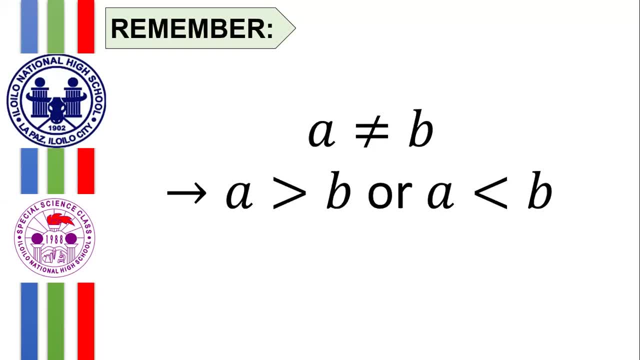 And we have to remember that in mathematics, if A is not equal to B, then it means either your A is greater than B or the first number, A, is less than B. So what I wanted to know, or what I wanted you to do, is that if there is a significant difference, 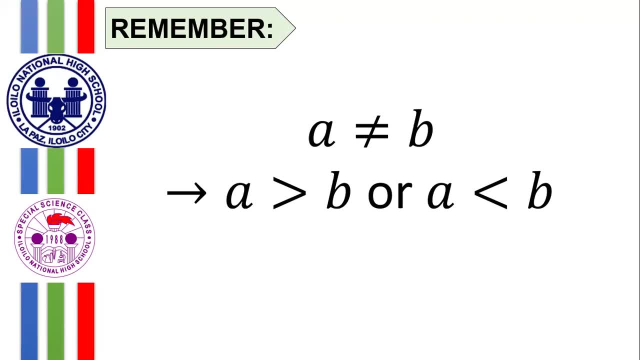 then you have to tell if one is larger than the second or the first is less than the second. And how do you do that? We have to examine their means for this case. So from here the mean of scholars is a 75.45, while that of non-scholars is 67.10.. For now, we will use that, the mean of, as basis for now. 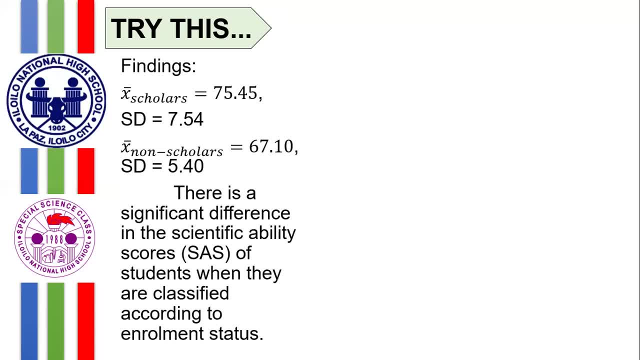 And here is our result. So a possible interpretation is: since they are not, there is a significant difference in their scientific ability, So therefore one of them is greater than significantly greater than the other, or significantly smaller than the other. So you just have to choose. 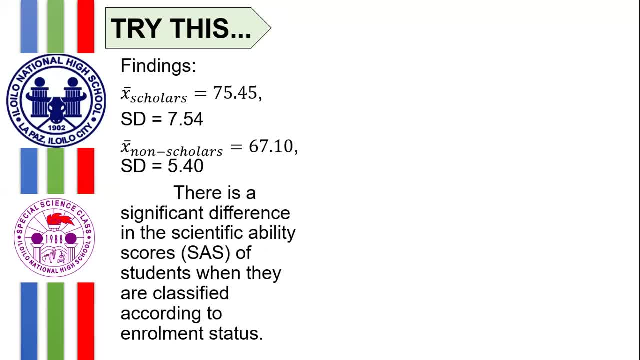 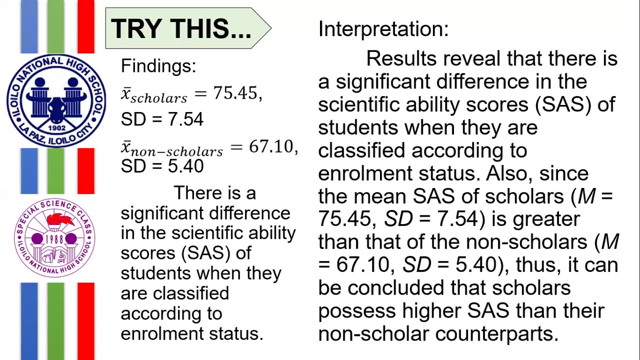 Which one you have to report: significantly greater than or significantly less than, or their other manifestations or their other ways of their synonyms, for example, could also be used. So for here, here's my possible interpretation. Results revealed with ED. results revealed that there is a significant difference in. 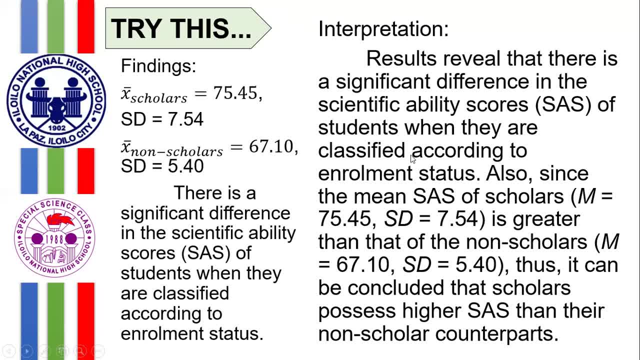 the scientific ability scores, or SAS, of students when they are classified according to enrollment status. So I just reiterated this Also. so if there's a significant difference, you have to examine their means. You see that the mean of scholars is 75.45, which is bigger than the mean. 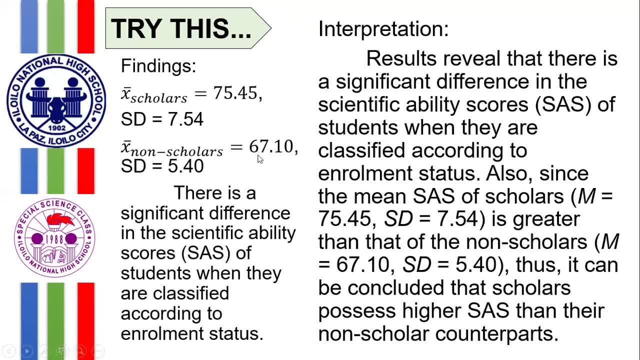 of scholars, which is 67.10.. By the way, it is a presumption here that the higher the score, the higher the scientific ability. the lower the score, the lower the scientific ability. for this context, And if you could see, since also since the mean SAS of scholars, then report the mean and 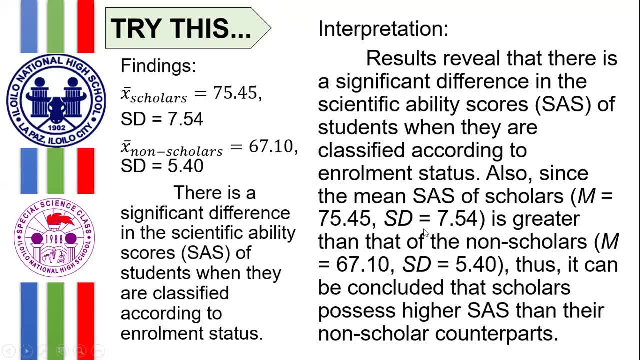 standard deviation. so M equals 75.45, ST 7.54, is greater than that of the non-scholars, M equals 67.10. And ST of 5.40. Thus it can be concluded that scholars possess higher SAS than the non-scholar. 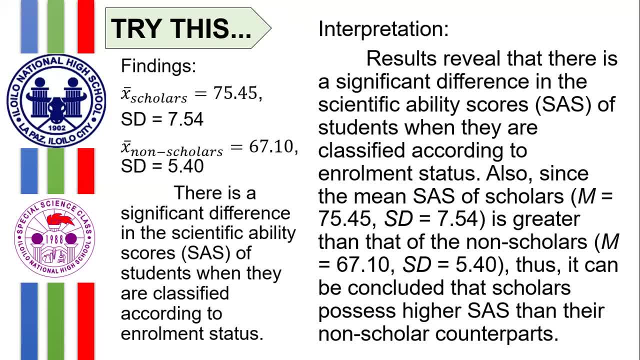 counterparts. So you see, for this particular case, I emphasized which one is higher than the other. Take note, take note of this: If there is no significant difference, then you treat them as equals. So they have similar, they are equal in terms. 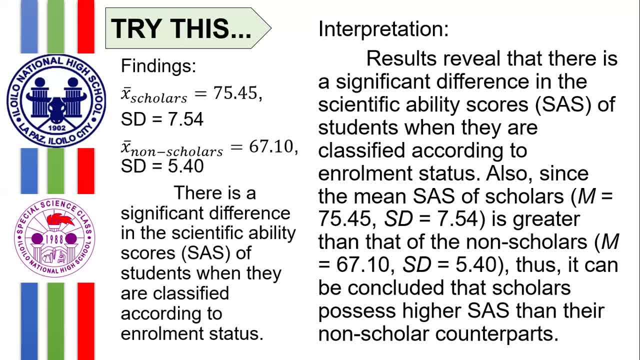 They are statistically equal in terms of a certain attribute, for example, But if there is a significant difference, I would like you to report which one is greater than the other and which one is smaller than the other, or I mean which one is smaller than the other. 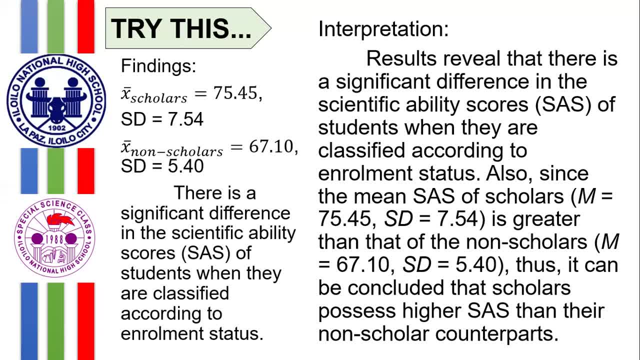 and you have to provide a higher interpretation of that. Okay, So that is for the second case, But if your other way, your way, is different from this, no problem. What's more important is that you capture the essence of the interpretation. 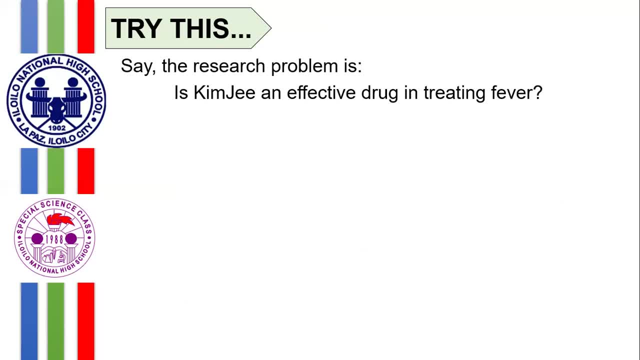 And how about for letter? for the last one Say: is CHEM-G an effective drug in treating fever? So let's say you before is, let's say you have participants and before they if they have a fever, with a mean of 38.50 degrees Celsius in terms of temperature, rather, 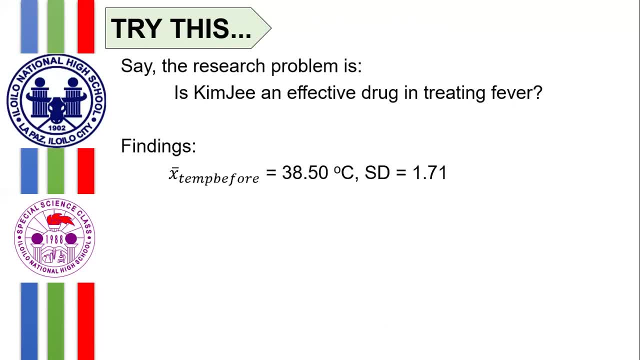 with a standard deviation of 1.71.. And supposing, after taking CHEM-G drug for, say, 24 hours, you took the temperature after, and the mean now is 37.01 degrees Celsius, with a standard deviation of 1.14.. And so you might ask, and I mean the results revealed, 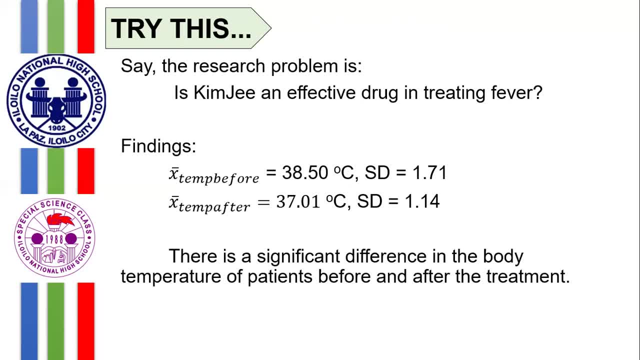 that there is a significant difference in the body temperature of patients before and after the treatment. significant difference, So what possible interpretation may be given to this? Take note: there's a significant difference here, So you have to report which one is greater than the. 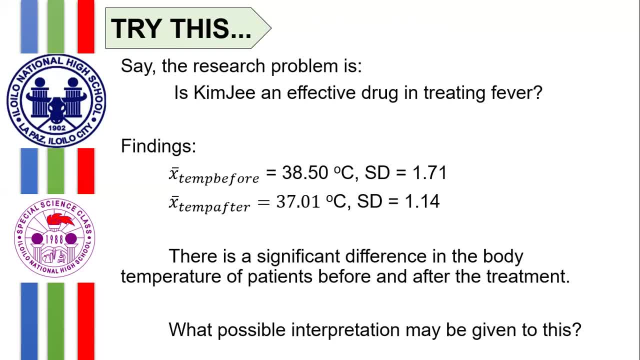 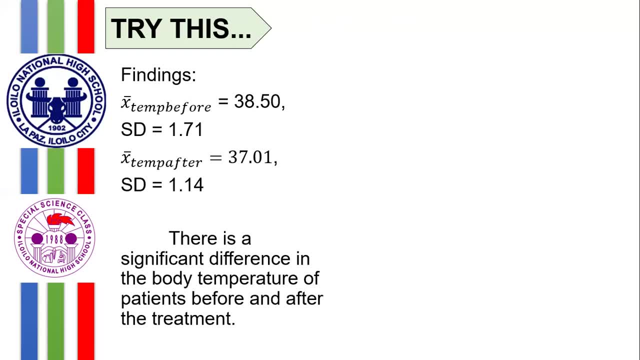 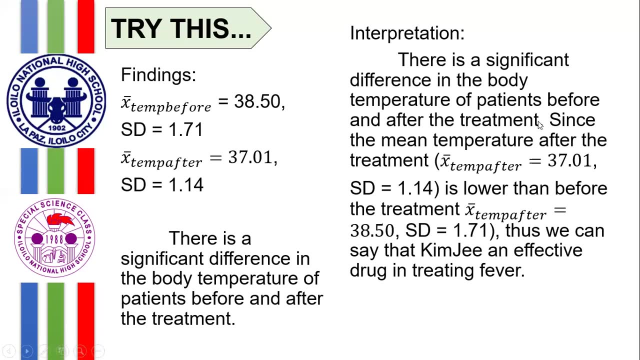 other, or which one is smaller than the other. And what do they mean In this case? since you could see from here that the temperature is lower, you could say there is a significant difference in the body temperature of patients before and after the treatment. So I just reiterated this And if you could see, since the mean temperature after the 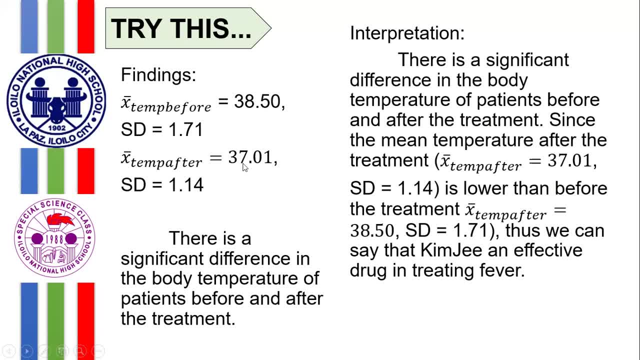 treatment. then you state the mean and standard deviations here is lower than that before of the treatment. then thus we can say that KimG is an effective drug in treating fever. How come you could claim effectively that KimG is an effective drug in treating fever? 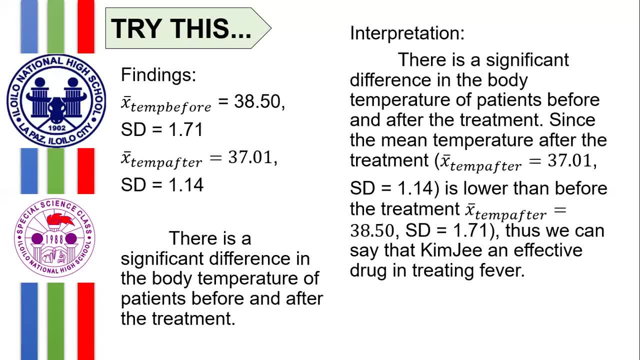 Because it was able to significantly lower temperature. It was able to decrease temperature that leads to a temperature that's nearly normal, for example. But if ever? there's no example? but what happens if there is no significant difference, If there's no significant?